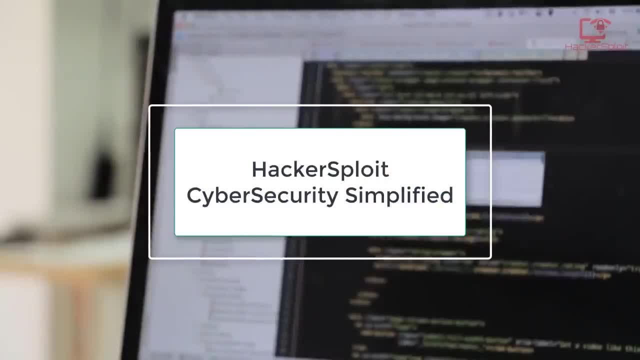 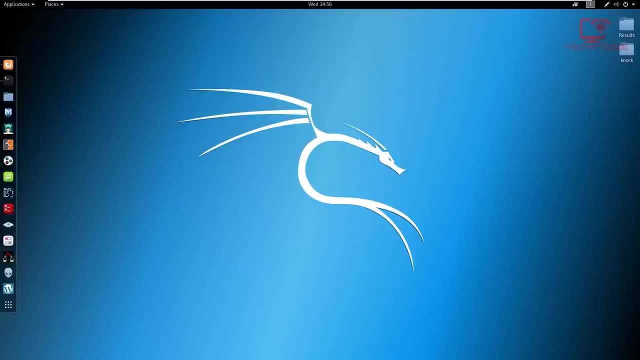 Hey guys, Hack Exploit here back again with another video and welcome to the web penetration testing series. we were going to be getting started with our first video. I know I've touched upon WordPress scan and stuff like that, But this is now, you know, taking you through the basics and 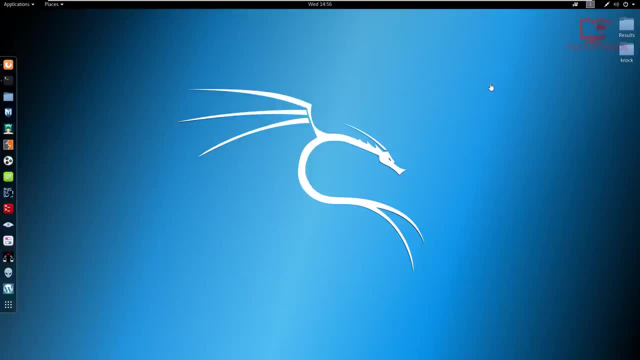 moving your way up. Alright, so for those of you asking about Hydra and the word lists, I will be uploading the word list to my website after upload this video. As for Hydra, Hydra belongs to the cracking, the cracking, the cracking section, which we'll be getting to, but you know. 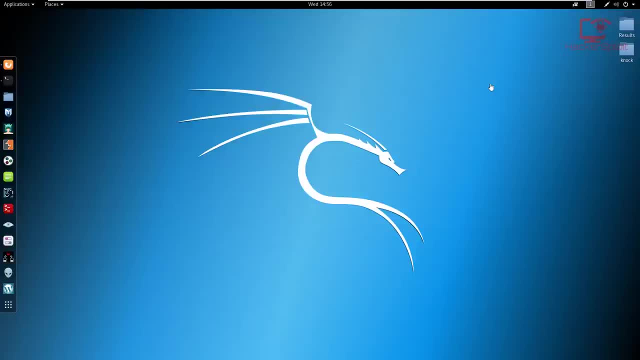 that's really focused on cracking services on ports and credentials. you know stuff like that, So it really doesn't come into play when we're talking about web penetration testing. Alright, so in this video we're going to be looking at Nick toe, which is a web vulnerability scanner. 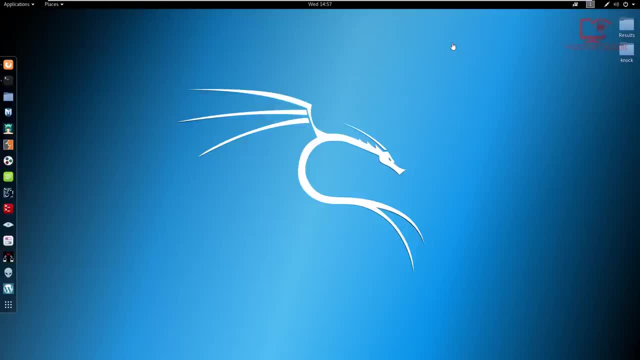 or a website. It's a website web server security scanner And it is, you know, it's fantastic for detecting vulnerabilities on the server. All right. Now the thing I like about Nick toe- and I use it a lot in the professional, you know, for professional. 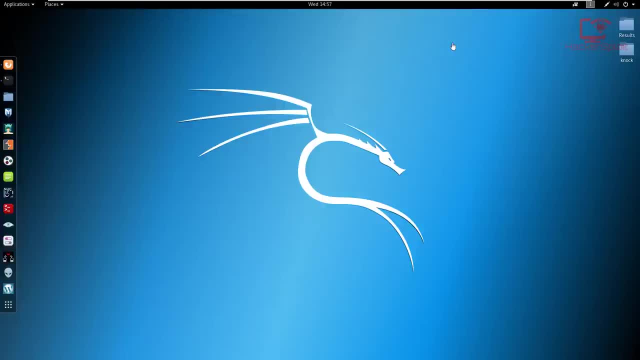 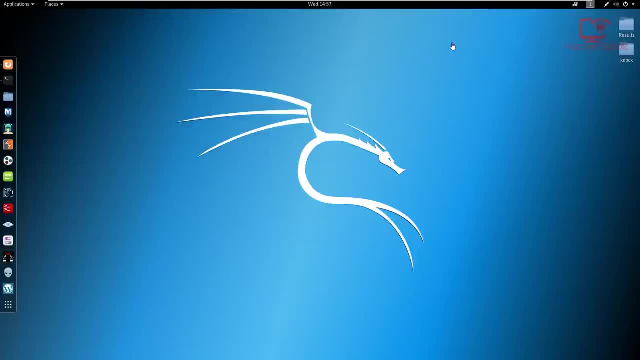 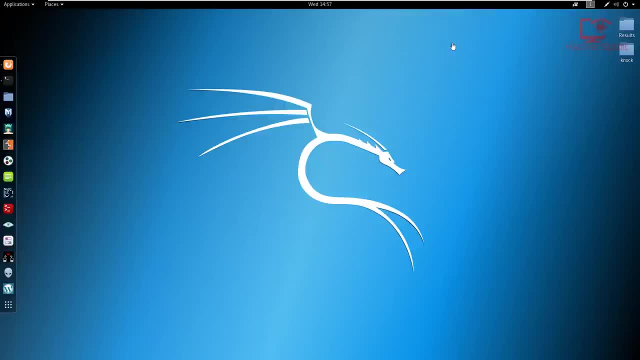 you know might sound a bit confusing to you if you're a beginner now, But when we'll be moving along, you know, using tools like burp suite, we'll get all. it will get into this really, really in depth, right. 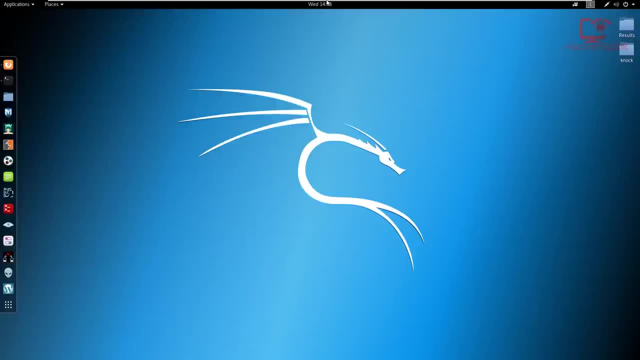 So let's get started. Now. I'm going to be using the web, the WordPress virtual machine or the WordPress server that we actually configured. So I've reset it again And it is using new credentials that I'm unaware of, but the IP address is still the same And I've opened it. 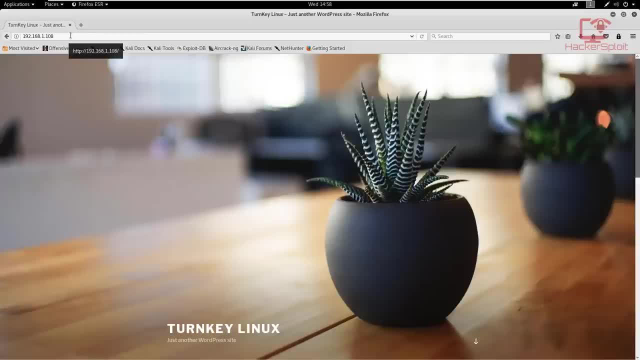 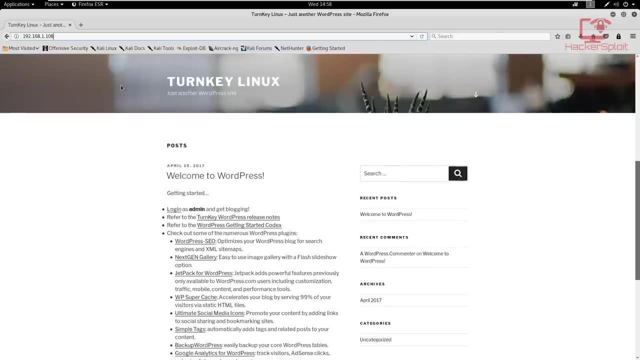 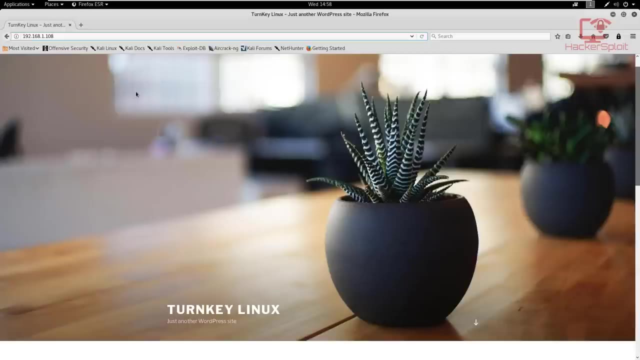 up on my, on my own Mozilla Firefox. There we are. that's the IP address: 192 point 168, point 1.108.. And it is indeed the WordPress site that is being hosted on the Debian server. Now, what I'm going to do is, as we move along, I'm going to actually log in to the WordPress site. 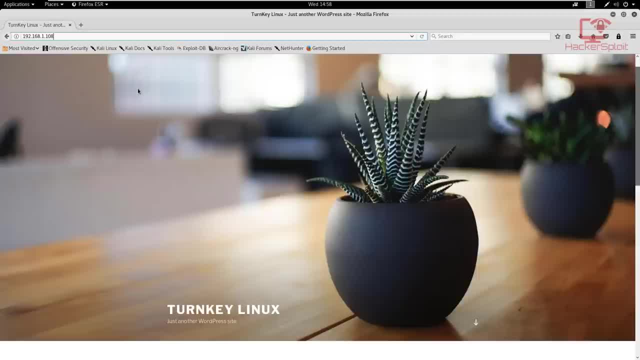 and I'm going to update the WordPress version and the plugins to make it more secure. That way it becomes a little bit more challenging, Alright, but for now we're going to be using- we're going to be looking at how to use Nikto Alright to scan for any vulnerabilities that we might find. 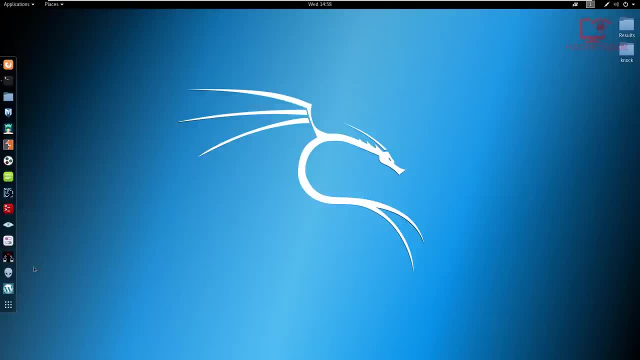 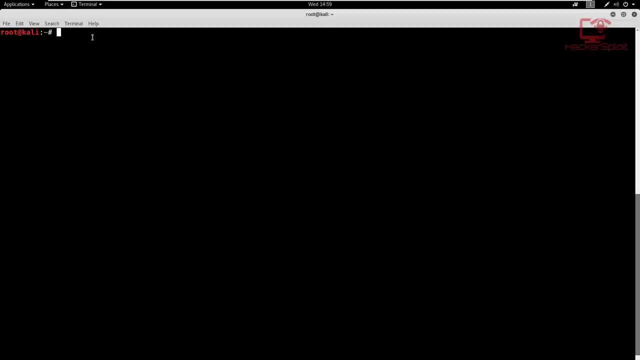 on the site. So, as you can see, I already have it locked to my favorites here on my dock because I use it quite a lot. But to launch it it's really very simple. Just open up your terminal and just hit in Nikto. Alright, now what I'm going to do is I'm 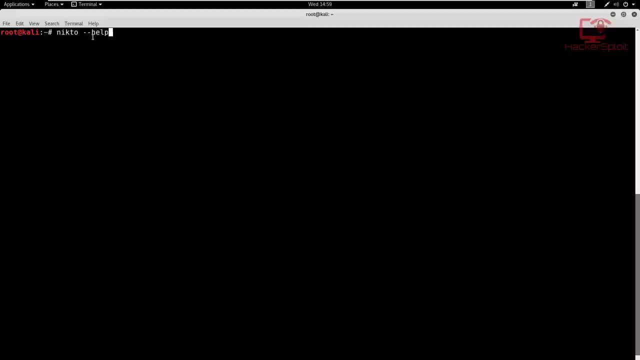 just going to open up the Help menu, because it is very, very important here, so that I can explain what each of the commands are and what they do, and, more specifically, the commands that we're going to be looking at in this video. Alright, so let me just open that up And, as you can see, 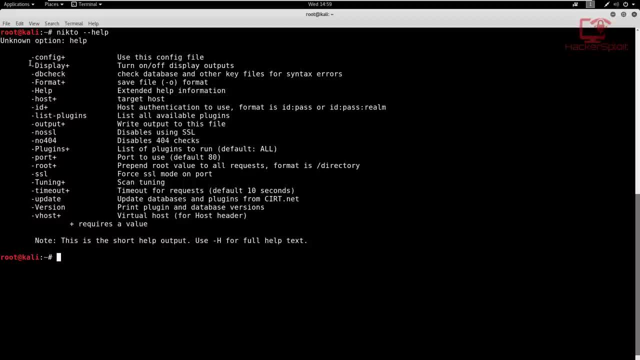 we've got from the right from the beginning, we can see that it's sorted really really well, And this is why I really like Nikto. Now some of you might be asking, or you might have this question in your mind. Well, 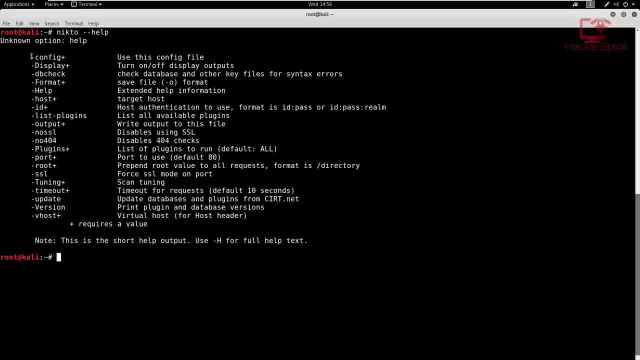 you showed us about WordPress scan, doesn't this just do the exact same thing? Well, WordPress scan is only designed to sniff out vulnerabilities on a WordPress website. The good thing about Nikto is it works on any web web server or website for that matter, And you know once. you know that. 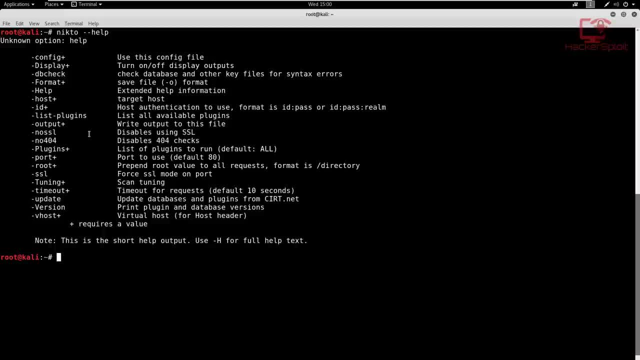 it's really, really fun, fantastic, because it works on any site or any web server, as we have already seen. So let's look at what these commands do Now. some of the most important commands are: the DB check, which checks for databases. the format, which allows us to change the output format. More. 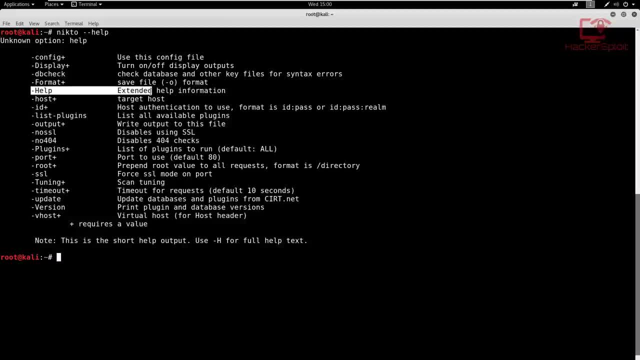 specifically the help, the help menu which is specified here, which is again is great because it gives you help. We then have the host. very, very important, allows you to select the host which, without this command, you would not be able to use Nikto. you're pretty much right, you then? 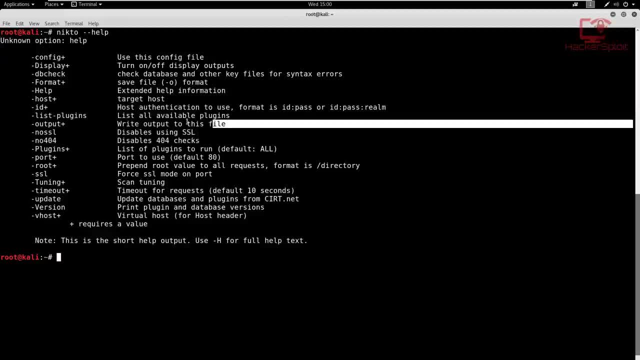 have plugins to list all the plugins, Alright, so let's look at what these commands do. So let's look at the plugins. you then have the output, which allows you to output your results into a file, are very, very important, if you're a penetration tester, to always have documentation of all the 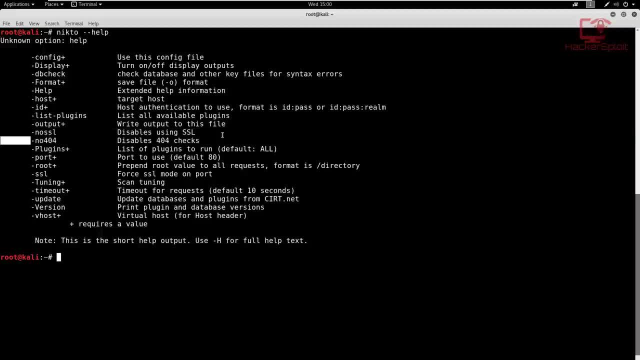 scans you're performing, you have no SSL which disable the using SSL. The port which you are going to be using in this video, we're going to be specifying to use the default port, which is port 80, which I'll show you how to specify. you can also change the port if you want, to which you 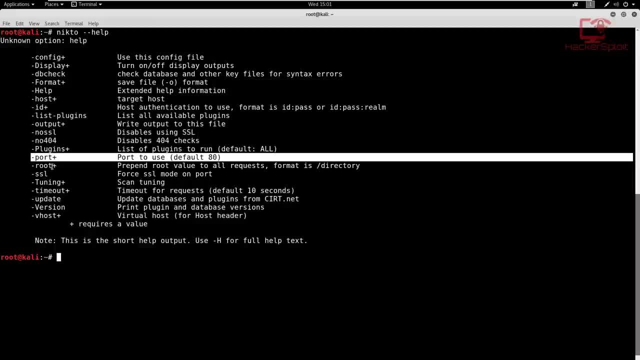 know would make a lot of sense. You're performing some serious scan that is more specialized. you then have your force SSL mode on the port, which is not that important- you don't come across that a lot- And you can update it And 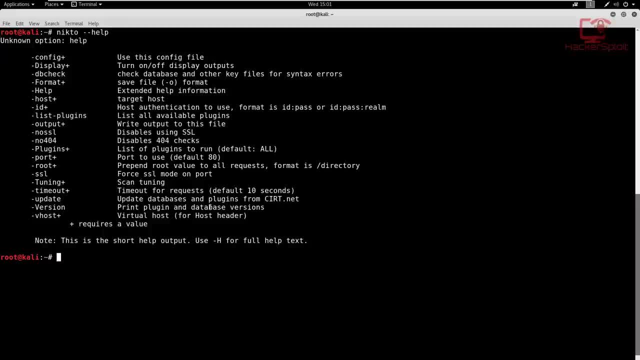 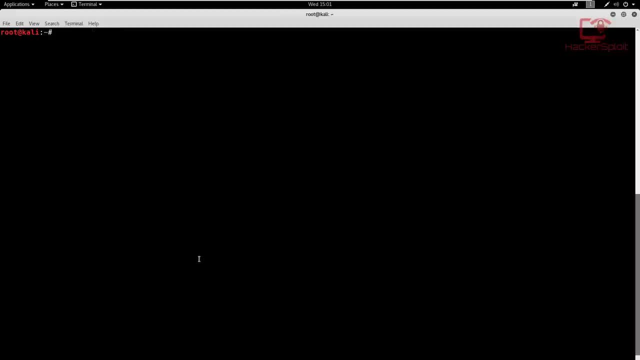 you can print the plugin and database versions if you want to. Alright, so let's get started with the commands that we're going to be using. So I'm just going to clear this out And we're going to get started now. So, if we remember correctly, we're going to use Nikto And to specify the host. 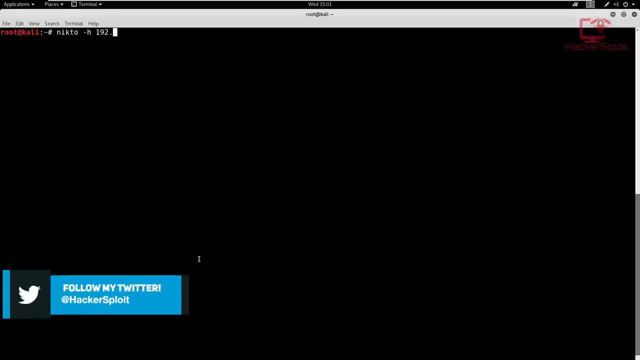 we use the H command, And after this I would use the. I would select the web, the website address, or the domain for that matter, or the IP addresses I'm going to be doing now. So 192.168, whoops. 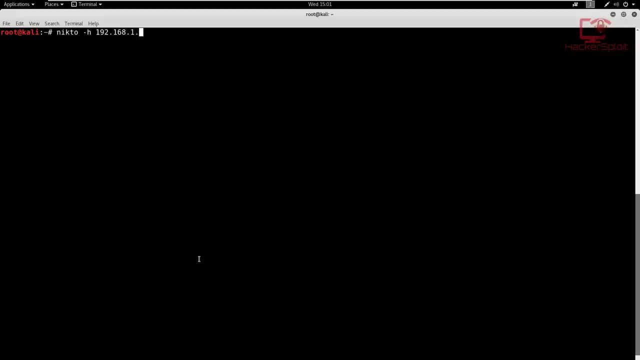 point 1.108.. And I've selected that. I've used the command, the H command, which means I'm using, that's the host. I now want to specify the port, which is the only other command that I'm going to be using. So we use the P. 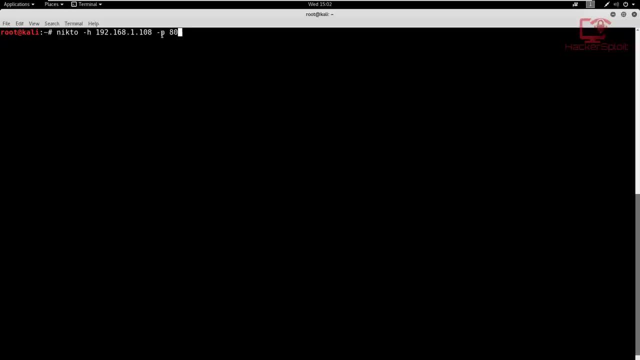 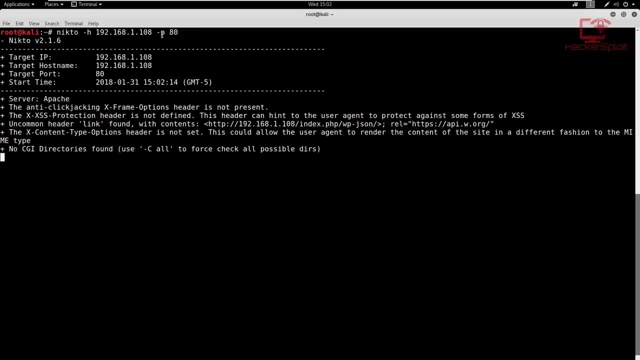 And the we're specifying the port, which is port 80.. And let's hit enter And let's see what vulnerabilities we can find here. Alright, so I'm going to hit enter And it's going to take the server, which is Apache, which we already know, as we've looked at this previously. And there we are. 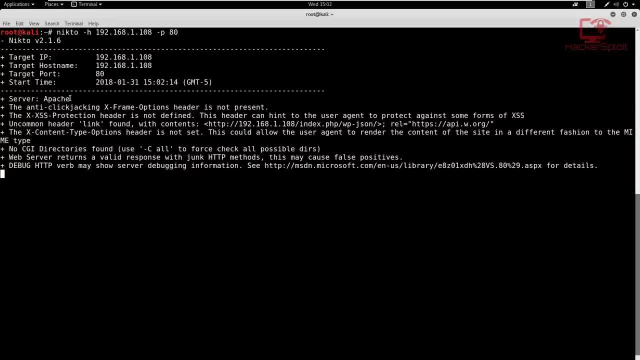 we've already got the cross. the cross site scripting protection header is not defined. that's a very, very huge vulnerability. we'll be looking at how to exploit all of these, the you know vulnerabilities like cross site scripting using tools like burp suite, and you know file upload vulnerabilities. 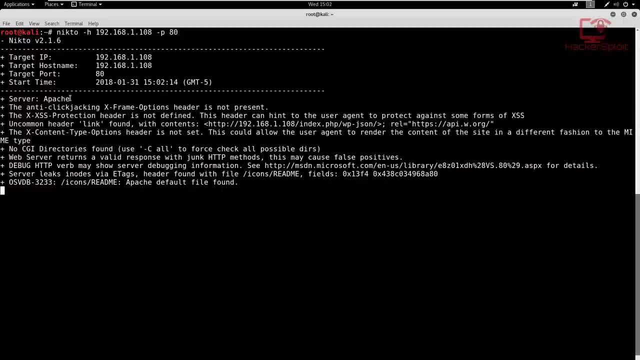 all of that good stuff, because a lot of you guys have been asking me about bug bounty hunting and how do I get started? Because you know, hacking on the web is a different ballgame. To be honest, it's quite tricky because every site is configured differently. Alright, so it's returned. 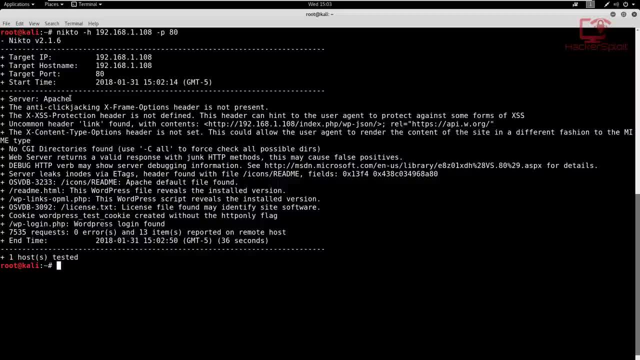 the results And you can look at all the vulnerabilities that it was able to find out. So the WordPress script. I reveals the installed version, which is, as you can see, that that looks like a CVE version cookie WordPress. So yeah, there's not a lot of important stuff that we were able to gather from. 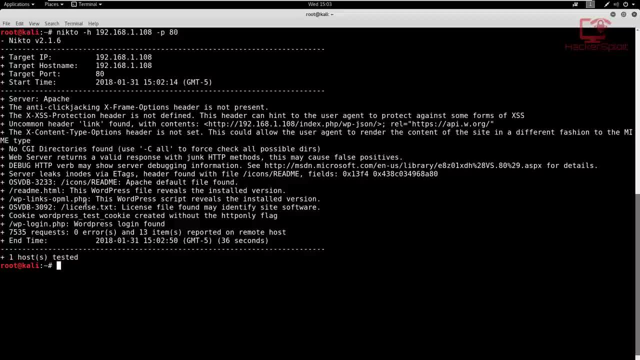 here Again, it would be much more wise to scan a WordPress site with WordPress scan, But for other websites this is fantastic. So that is how to scan for vulnerabilities that exist on a web server. In this case, I work WordPress site. Now let's look at one more command. 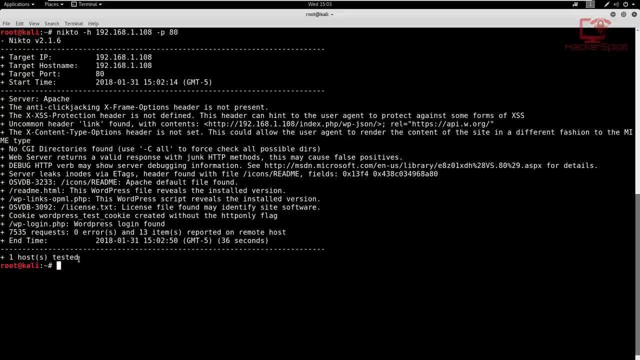 which is the output command, which is very, very important. So we're going to try and output this on the desktop. So I'm just going to change my directory to my desktop, So like so, and let me just clear the terminal. So we're going to use the same command, which is Nikto H, which is the 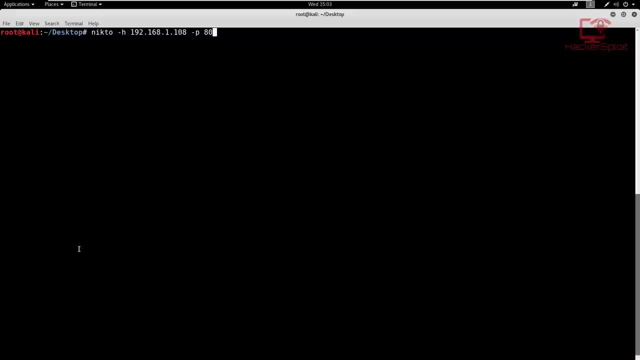 host: 192.168.1.108.. We're specifying the port, which is port 80.. And now we have to specify the fact that we are using the output command. So, Oh, and we specify the file name, which we're going to say is: let's see, Hmm, let's just call it. 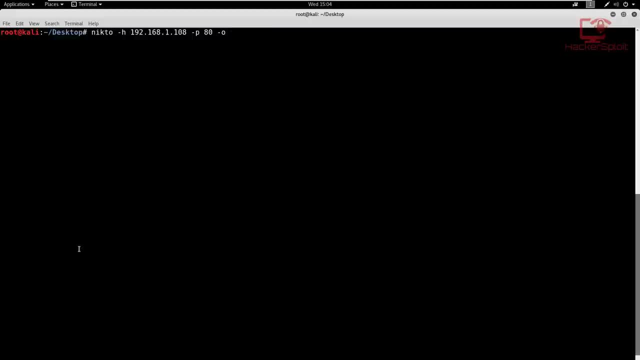 results. Let's just call it Nikto results Results. always good to name your, your documentation appropriately. And now we want to specify the file type, which in this case we can just say: we use the command F, capital F, to specify the file type of the file extension In. 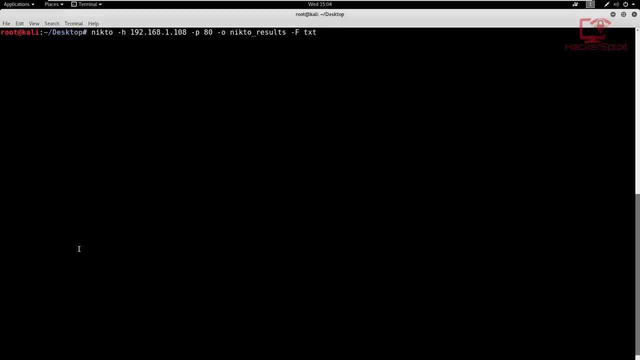 this case, we're going to specify the file type, which, in this case, we're going to specify the file type of the file extension. In this case, I'm just going to select dot txt, just to keep things basic, and I'm going to hit enter is going to start the scanning process And once the 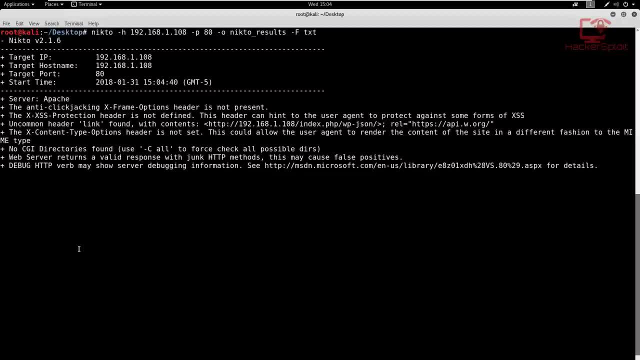 scanning process is complete, it's going to save- it's actually saving- the data right now, in real time, as it's performing the scan Alright, so just give it a few seconds to complete the scan and we'll be able to see whether or not the information was stored in the file that we 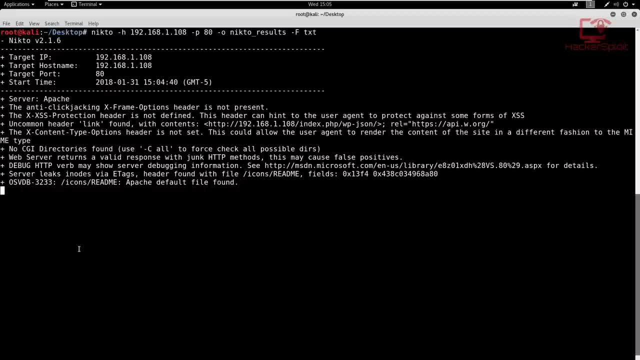 specified it to be stored in. Alright, we'll be looking at all of these vulnerabilities as we, as we move along. But the first thing is to understand what we've got and how to gather information about a web server or website, And this is the basic, you know, just getting started. 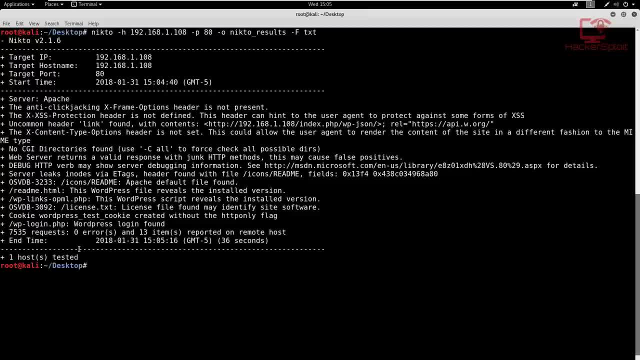 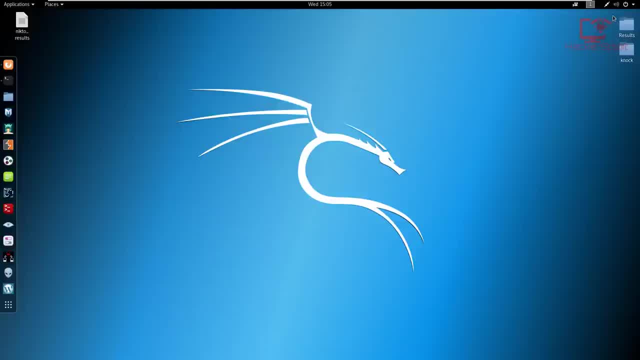 with it. It's very, very good to get accustomed to the tools. Alright, so, as you can see, it's completed And if we just check the desktop here, we have the NICTO results there. we are Fantastic If I just opened up the file and it has stored all the information very, very. 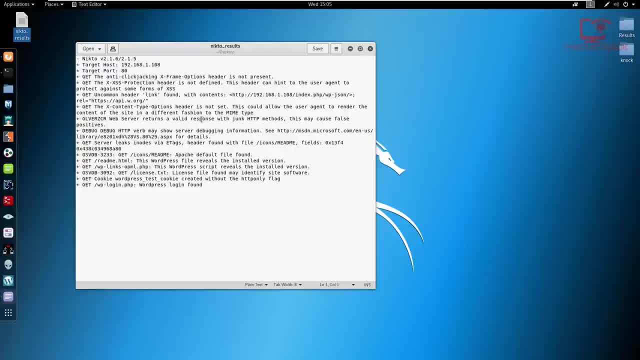 important that you store this information. it acts as a good way to save your data And, if you want to get a good way of of showing, or it acts as documentation, and that is very important, especially for a penetration tester. Alright, so that is going to be it for NICTO. we'll be moving. 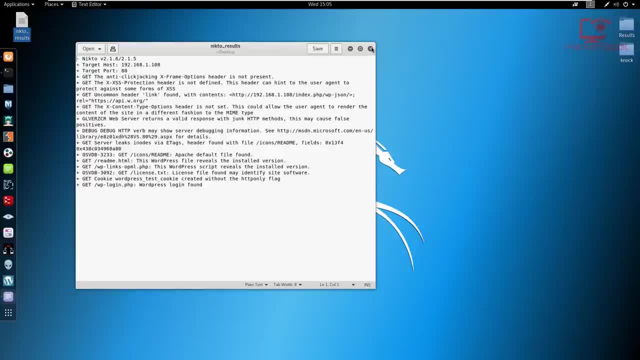 along swiftly after this And we know we'll be looking at cross site scripting, how to use burp suite, all of the great stuff Alright. so I want you guys to stay tuned for that. So that's going to be it for this video, guys. I hope you guys found value in this video. If you did, please. 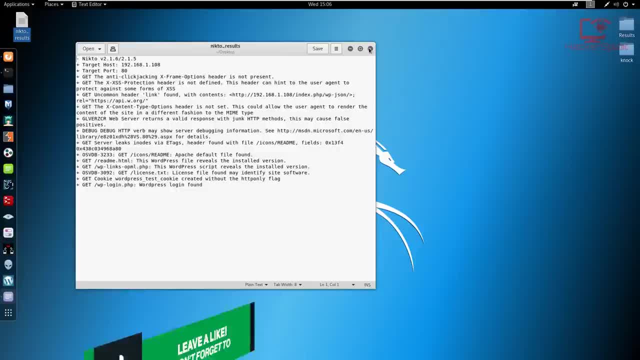 leave a like down below. If you have any questions- any at all- hit me up on my social networks or or, you know more specifically, you can hit me up in the comment section. If you have any personal questions, please hit me up on. kick One more thing by the. 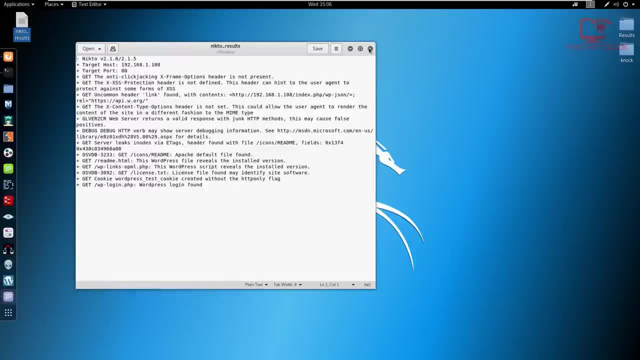 way, if I do not reply to your comment or question, it doesn't mean that I do not want to. it's because there are a lot of these comments and I have to go through them as much as I can And I tried to reply to all of them because the comments are increasing as the channel is increasing And 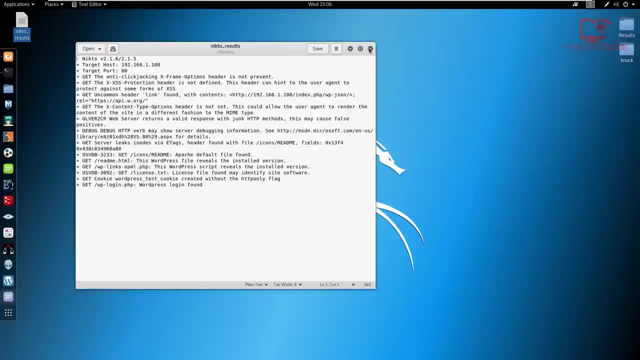 you know, if I don't reply to your message, please don't take in the wrong way. I will reply. just give me a. you know up to or two days at the latest. I just want to thank you for all the support, guys. Thank you for. 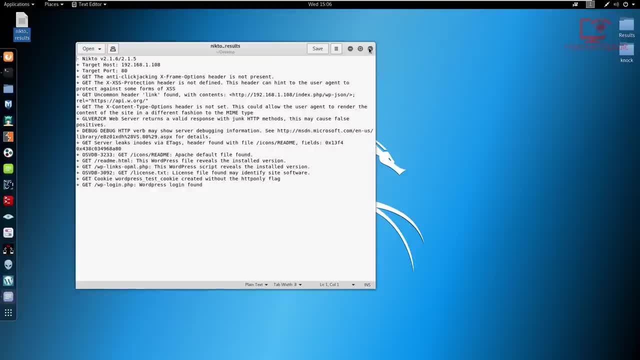 supporting me, and I have something really, really important that I want to announce soon For those of you who are watching the video till now. you know, stay tuned for that And, yeah, I'll be seeing you in the next video. Peace. Subtitles by the Amaraorg community. 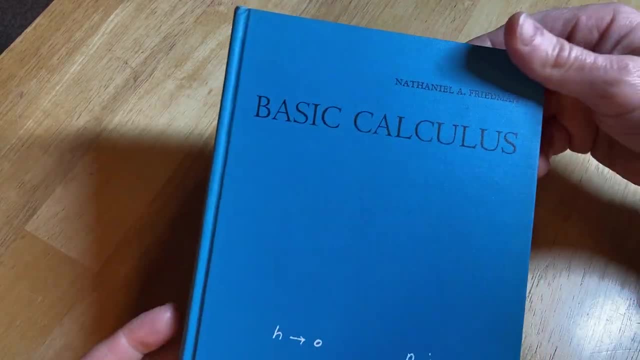 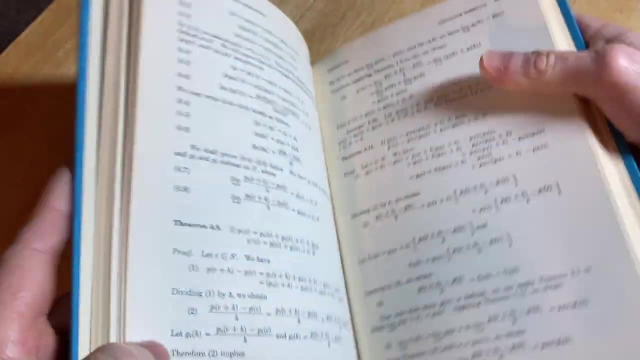 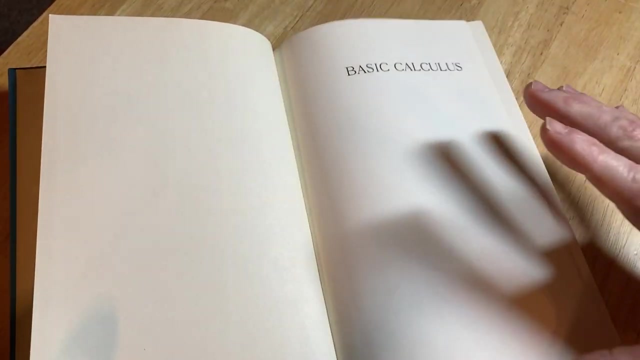 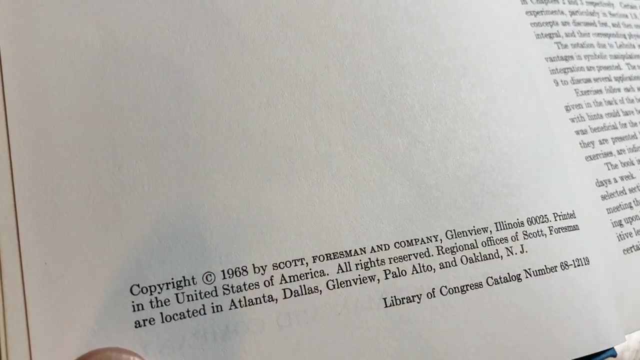 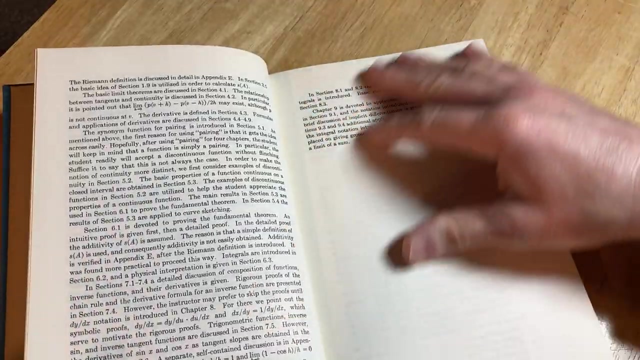 Here we have a book called Basic Calculus. It was written by Nathaniel Friedman and this is a book. I've actually read portions of this book and worked through some of the examples. Basic Calculus is just an interesting book to look at 1968. It talks about the book. 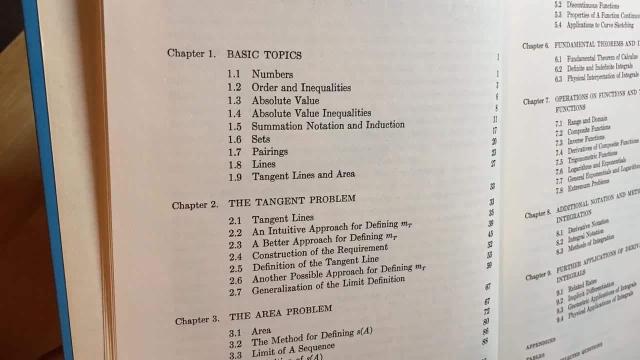 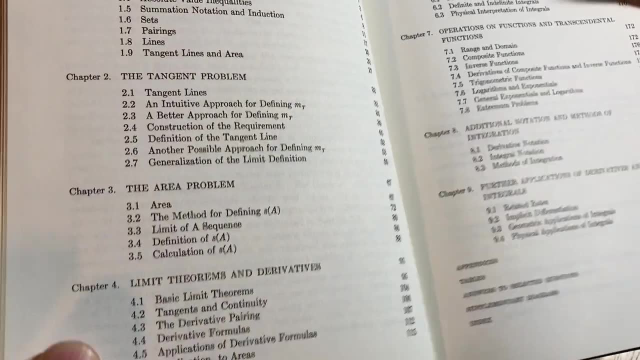 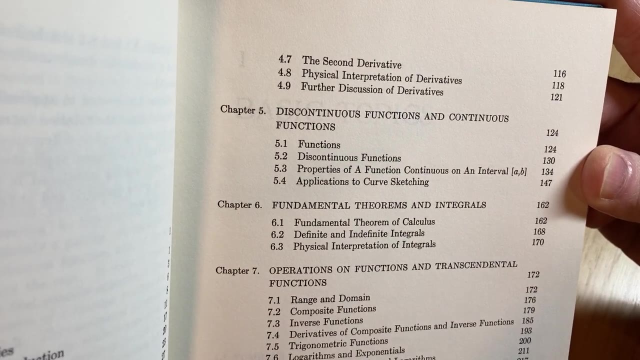 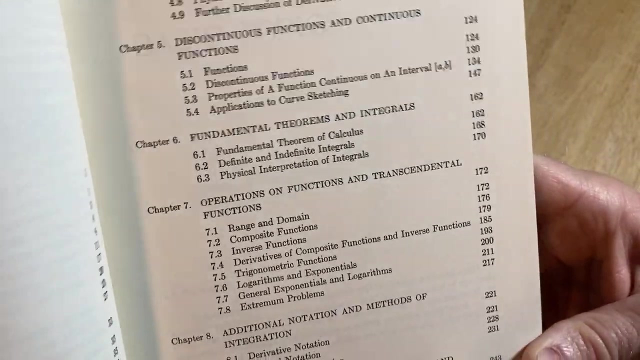 And then here we have the book. Here's the contents: Basic Topics: Tangent Problem Area, Problem Limit, Theorems and Derivatives, Discontinuous Functions and Continuous Functions, Properties of a Function Continuous on Interval AB, so Closed Interval. Fundamental Theorems and Integrals, so the Fundamental Theorem. 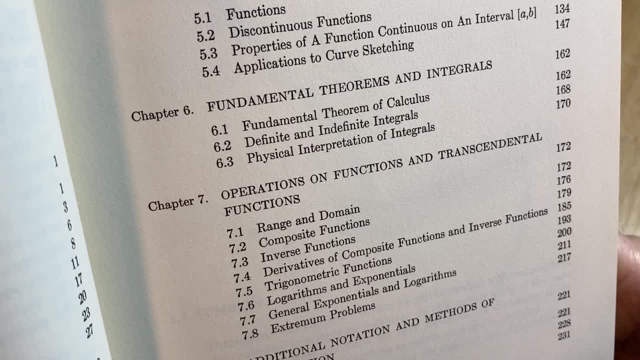 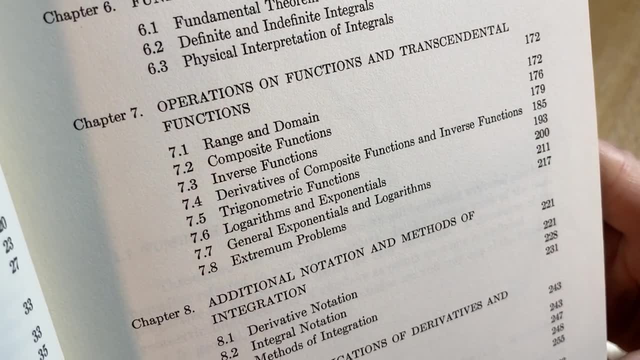 of Calculus, Definite and Indefinite Integrals, Physical Interpretation of Integrals, Operations on Functions and Transcendental Functions. So the Fundamental Theorem of Calculus, Definite and Indefinite Integrals, Physical Interpretation of Integrals, Additional Notation and Methods of Integration. Further,